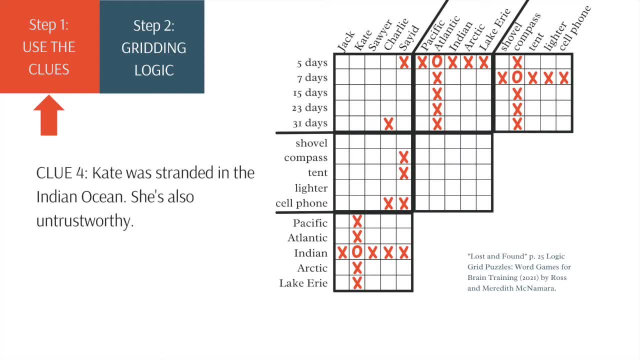 like untrustworthiness. In other words, this information is irrelevant. To complete the grid, just ignore it. Authors mention it. Well, it might be a funny reference to a different type of logic puzzle where some characters always tell the truth and others don't. Humor is always tricky. It doesn't. 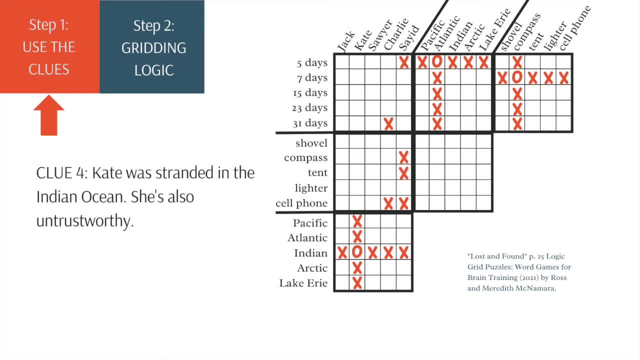 matter what joke you tell, There's always people who don't think it's funny. Personally, I try to avoid humor. Sorry, I'm kind of cracking myself up there. Okay, clue 5.. This is a big clue. It starts. 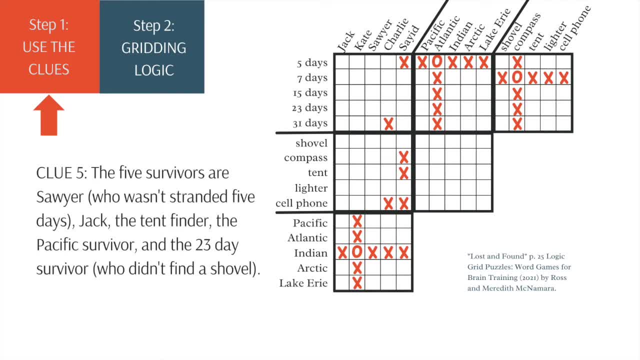 the five survivors are. That means each phrase applies to a different person. Sawyer, Jack, Tent Finder, Pacific Survivor 23-Day Survivor. Obviously, Sawyer is not Jack, We know that. But also Sawyer is not the Tent Finder or the 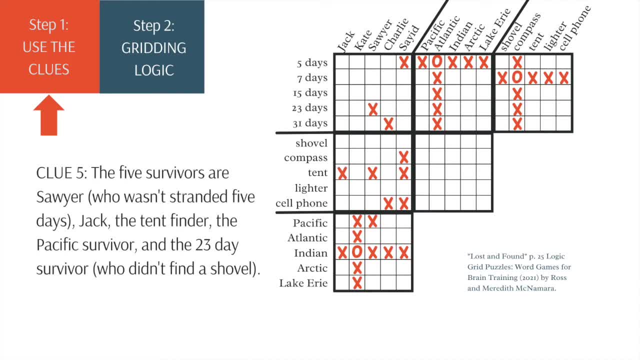 Pacific Survivor or the 23-Day Survivor. Jack is not the Tent Finder or the Pacific Survivor or the 23-Day Survivor. The Tent Finder is not the Pacific Survivor or the 23-Day Survivor, And the Pacific Survivor is not the 23-Day Survivor. And the clue also tells us that Sawyer isn't the five. 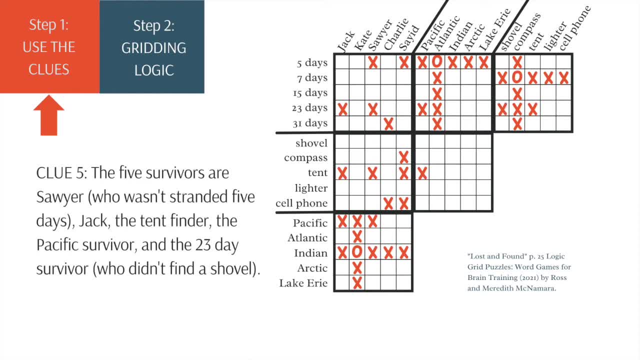 day survivor and the 23-day survivor isn't the shovel finder Clue. 6. Sawyer found a lighter and is very likable once you get to know him. Which trait helps you complete the grid? The lighter? Ah, now we know Saeed found the shovel Clue. 7. The Arctic person spent more time than the Lake. 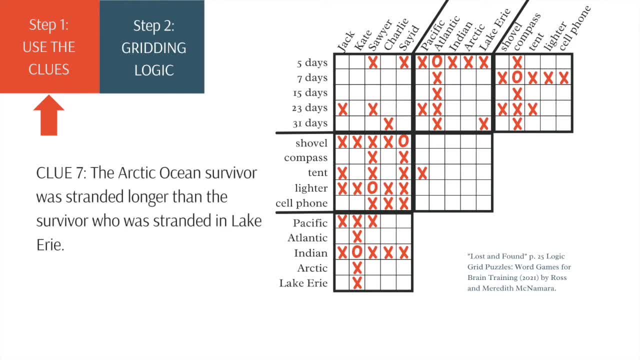 Erie person, so the Lake Erie person didn't spend the most time. Last clue: The shovel person spent less time than the lighter person, so the shovel person didn't spend the most time and the lighter person didn't spend the least time. Okay, that's what we get from the clues, but the puzzle's not. 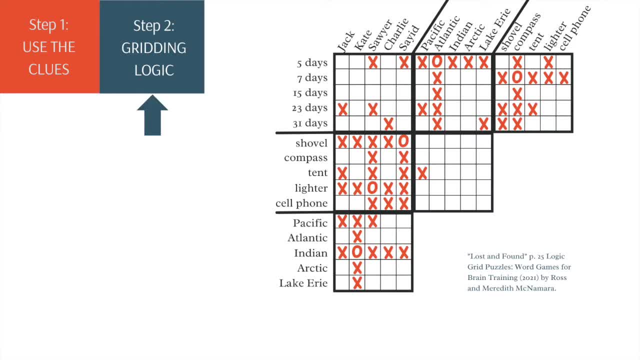 done. Now we need to use logic based just on the grid, Gridding logic. Let's start with Kate. She's in the Indian Ocean and she didn't find a shovel or a lighter. So the person in the Indian Ocean didn't find a shovel or a lighter. How about Sawyer? He found the lighter and he didn't spend. 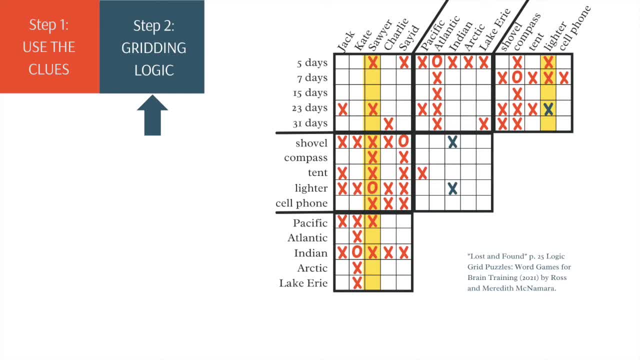 five or twenty-three days, So the lighter finder didn't spend five or twenty-three days. He also wasn't in the Pacific or the Atlantic, so the lighter finder wasn't in those places. Let's look at Saeed. He found the. 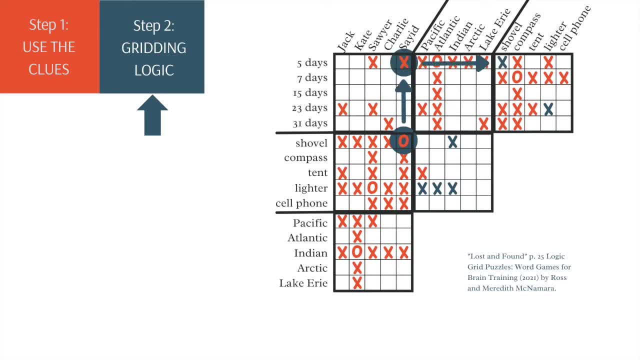 shovel and the shovel finder didn't spend five days, So that's fifteen days for the shovel finder plus all the X's for the items he didn't find. We also know the shovel finder, the fifteen day person and Saeed were the same person, So fifteen days for Saeed. Oh, and look up here. 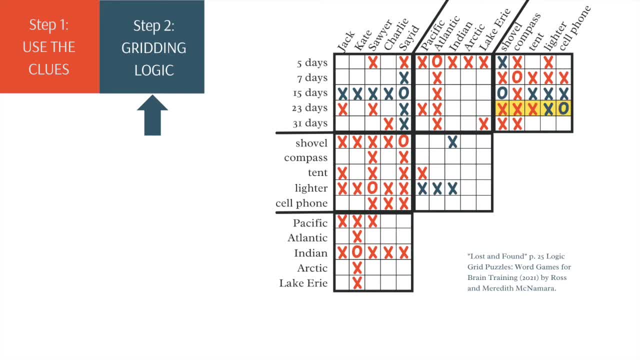 All X's except one blank. The twenty-three day person found the cell phone. That means the tent finder spent five days and the lighter finder spent thirty-one. Who is that lighter finder? We know already: It's Sawyer. Sawyer spent thirty-one days. That means he wasn't in the 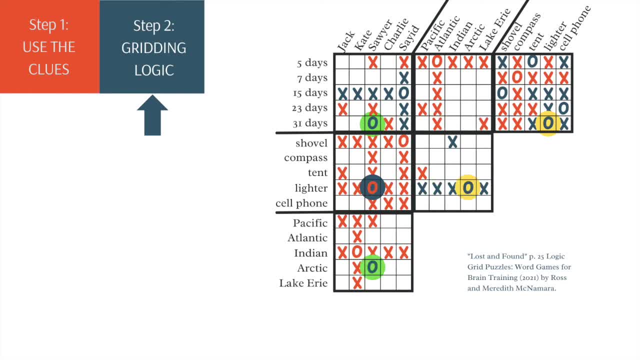 Atlantic or Lake Erie. so Sawyer was in the Arctic Ocean and therefore he was there for thirty-one days. Notice, we now know everything there is to know about Sawyer. Let's look at Saeed again: He spent fifteen days, so he wasn't in the Atlantic, Since he also wasn't in the Indian Ocean. 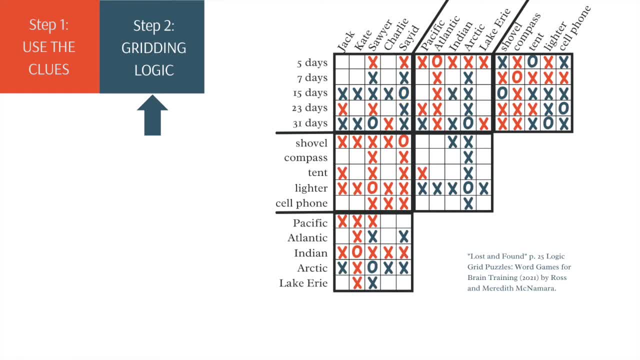 Indian Ocean and fifteen gets an X. What about the Atlantic person? Well, they found the tent, so they weren't Jack. so the five-day person wasn't Jack. Jack spent seven days Since the five-day person was in the Atlantic. they aren't Kate, so they're Charlie. That puts Saeed in the 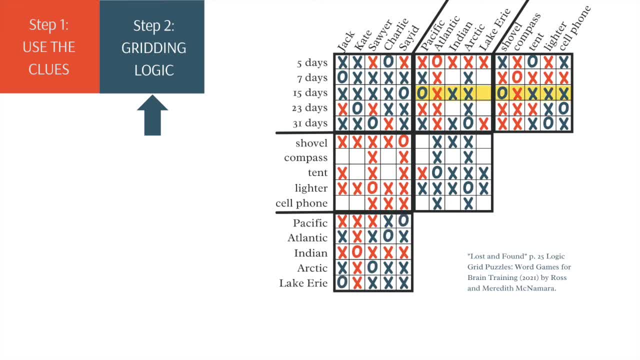 Pacific and Jack in Lake Erie Said in the Pacific found the shovel and Jack was the 7-day person who found the compass, so 7 days goes with Lake Erie. At this point we know the solution because we've identified every combination.